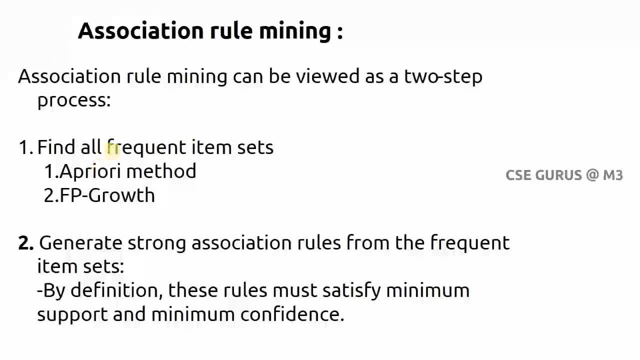 It is reviewed as a two step process. In the first step, that is finding all the frequent item sets. Second one is generating strong association rules from frequent item sets. So in the first step of association rule mining, you need to find all frequent item sets. How you can find means, there are two methods Again, one is a priori method, other one is FP growth. So now we can understand: a priori algorithm is useful for finding all frequent item sets. So for finding all frequent item sets, 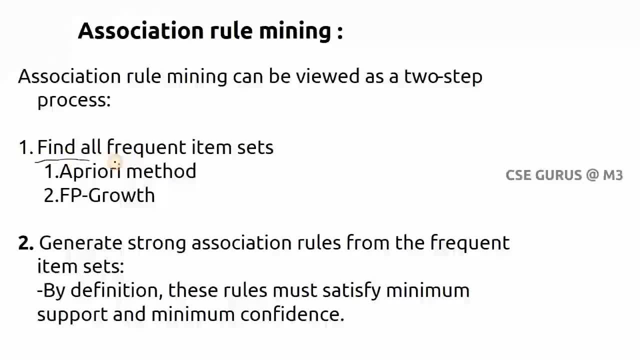 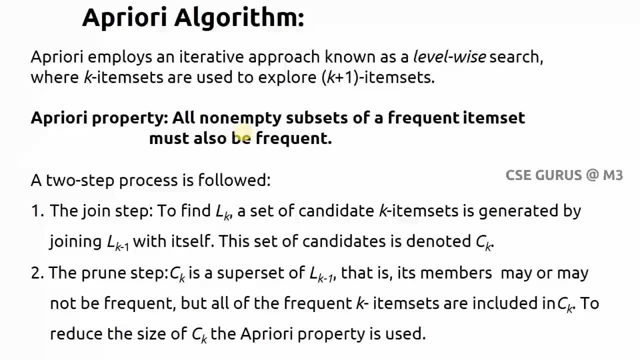 Remember this point. Now we will go for the a priori algorithm. So instead of going first to this theory part, I will explain this a priori algorithm with an example. After that we will come here and we will understand what is this, all those things. But remember this: a priori property, that is, all non empty subsets of a frequent item set must also be frequent. And especially, we will have again two steps, that is, join step and prune step. We will have join step and prune step. 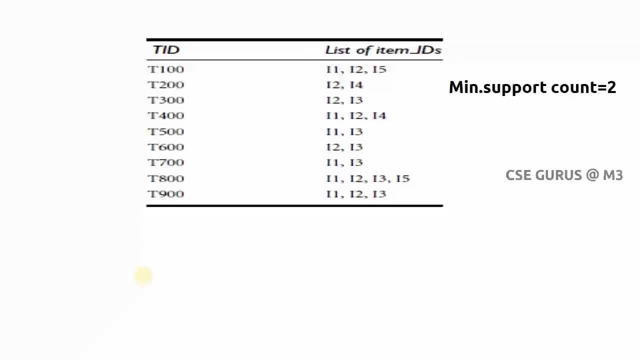 Prune step. Remember this point. So let us consider one database here, which consisting nine transactions, where, in each transactions, what are the list of items that are purchased by customers? So in the first transaction, three items are purchased, That is, I1, I2, I5.. In the second, I2, I4. like this you have all the transactions. Now the question is asked: like find all the frequent item sets by using a priori algorithm? 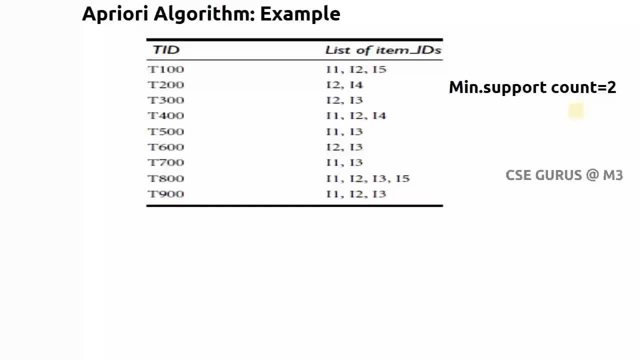 Where the minimum support is given as two, That is, minimum support count is given as two. So how to process this and how we can find the frequent item sets here. So we will see this. What is our first step? So here you can see: scan the D. D means database, Scan the database for count of each candidate, Candidate in the sense, each product. here you can see. So how many products are there? Totally five products: I1, I2, I3, I4, I5. So scan the database. That means 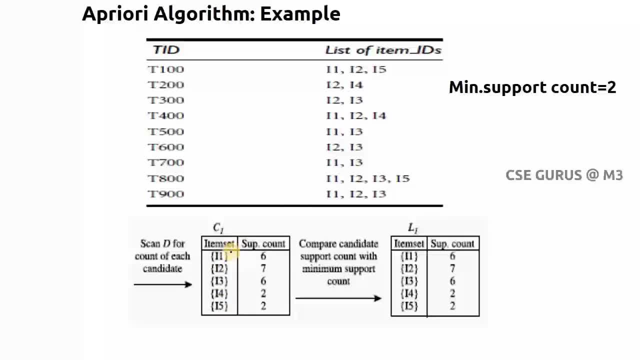 you need to find count of each items. That means that count we call it as support count. So for I1, how many transactions consisting of I1, you can check it. The total count is 1,, 2,, 3,, 4,, 5, 6.. I1 count is 6.. Like this we can write: What about I2?? So how many transactions consisting I2? So 7.. Like this: I3,, 6, I4, 2, I5. Again 2. Like this you need to write: and this we call it as C suffix: 1.. 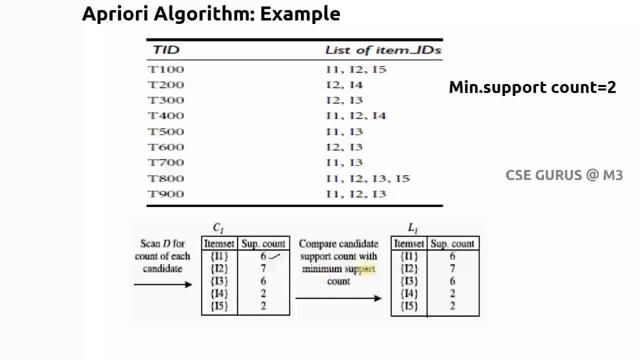 Now the next step is compare candidate support count with minimum support count. What is the minimum support count is given to? So compare it. That means compare in this support count. Of course. here we call this C1 as also one frequent item set. We call it as one frequent. Why we call it as one frequent means in each record, in each line, you can see only one item is there. That's why this is one frequent. Anyway, in the next we will find two frequent, after that three frequent. 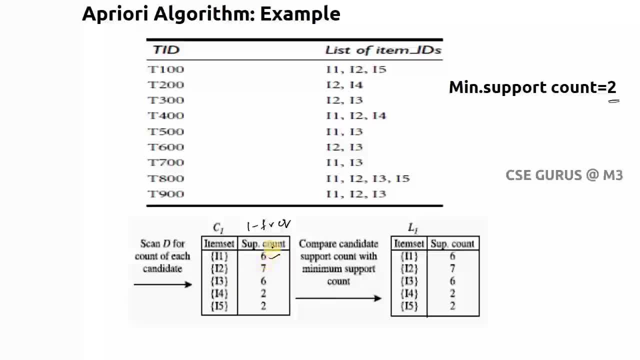 Like that, after finding support count in one frequent item sets. Now you need to compare with the minimum support count, that is 2.. So how many items are satisfying this minimum support count? If you observe, all the items are satisfying the minimum support count. So at least 2 should be the support count. So all are satisfying. Write all those things, Whatever the item sets are satisfying that you need to write here. So now this will become L suffix, 1.. You have taken 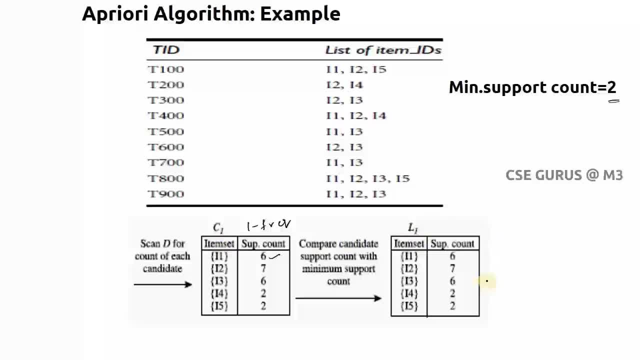 C1, then you are getting L1 from C1.. After that you need to find C2 from L1.. After that you need to find L2, like this. After that you need to find C3 from L2, like this, So up to: if you find that total records are empty, you need to do like this. So now, after L1, you need to find C2.. What is C2 actually? So C1 means one frequent item set. C2 means you need to generate two frequent item set. You need to generate two frequent item set. 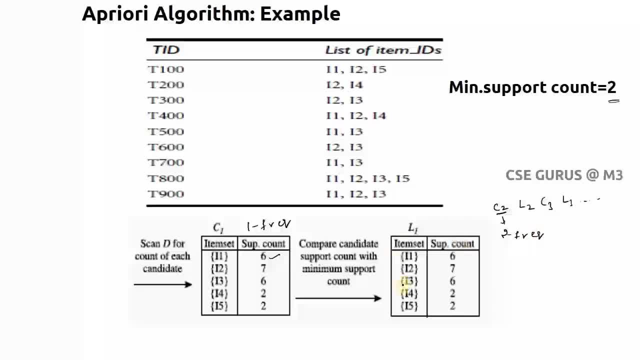 So what is this? two frequent means From L1. you need to make joins of two frequent Joins in the sense I will make one join, that is I1, I2.. Another join, I1, I3, like this. So I am writing here: I1, I2 is a one join, I1, I3. Next I1, I4.. I1, I5. From I2, I1 can I write: See, I2, I1 is also equals to I1, I2.. So I cannot write I2, I1. 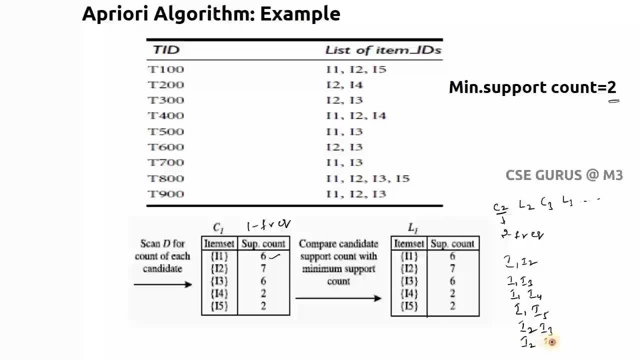 I2, I3, I can write. Next I2, I4, I can write. Next I2, I5, I can write. So next, what about I3, I1? I1, I3 is there, So I3, I2, I2, I3 is there, So I can write I3, I4, I3, I5. So final one, I4, I5.. So like this, I need to generate these things. you call them as two frequent item sets. All these things are. you call them as two frequent item sets? 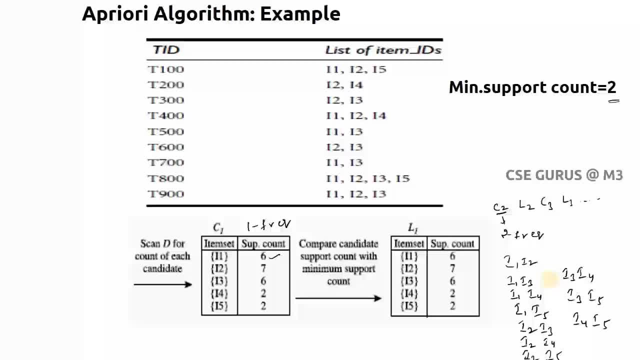 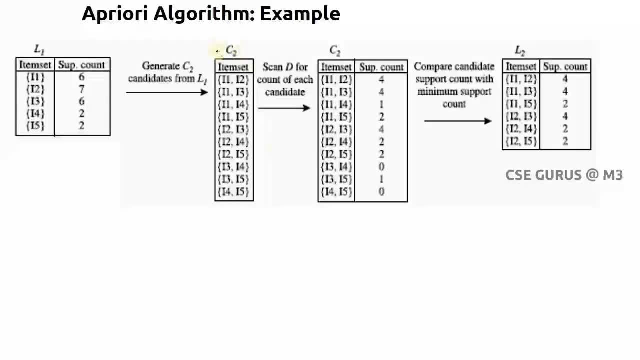 So now you need to write these two frequent item sets. You call it as C2.. Here you can observe. This is this part you can observe. C2 means all the two frequent item sets. I am writing here Two frequent item sets. 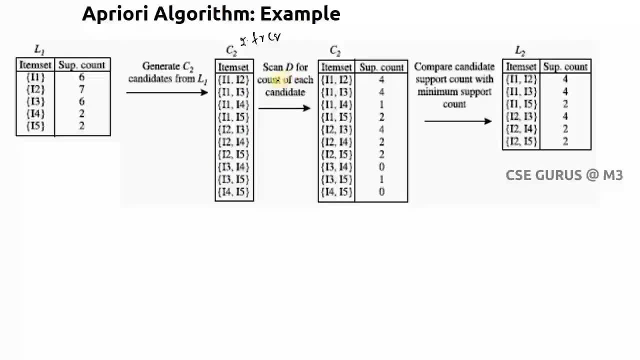 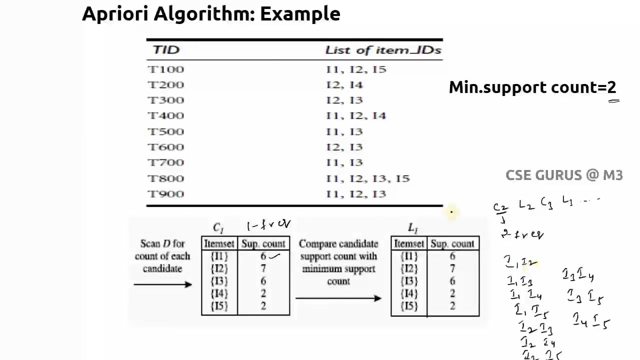 Now, after getting two frequent item sets and find again the same thing, that is, to scan the database count of each candidate, After finding this for C2, support count, you need to write What is the support count Here the count should be taken for each item set. That means how many transactions consisting of I1 as well as I2.. Let me take this example here. So I1, I2. I have written So how many transactions consisting both I1, I2? This is the one transaction. second, and here I1, is there no I2.. Here also no I2.. I cannot consider Here I1, I2,. third transaction here: 4.. So totally I1, I2, the support count will be 4.. 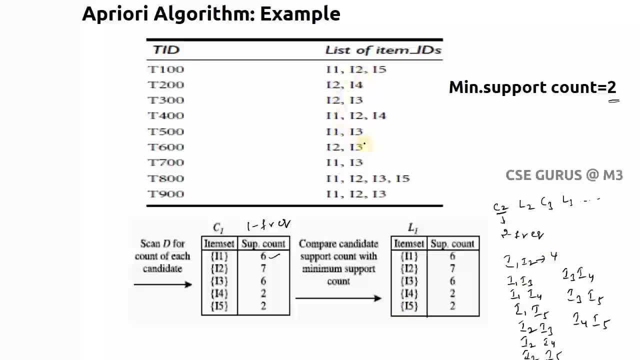 What about I1, I3?? So I1 and I3.. 1, 2, I1 and I3, I1 and I3, 4.. So irrespective of whether other transactions, other items are there or not, we cannot check that one Now. I1, I4.. So I1, I4, I1 and I4.. This is the one transaction, only one transaction. 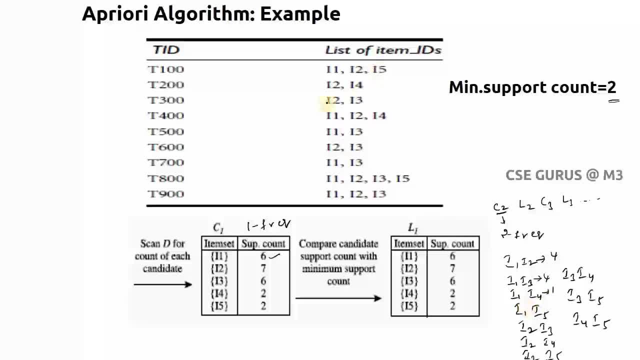 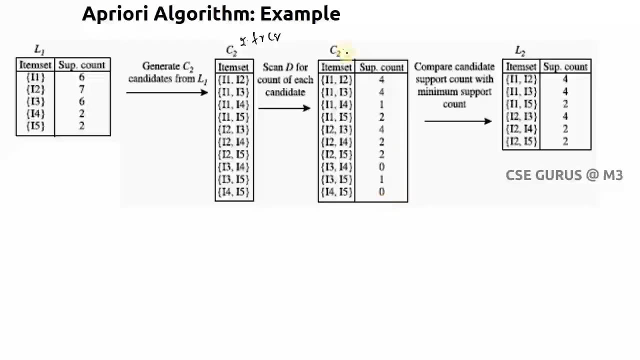 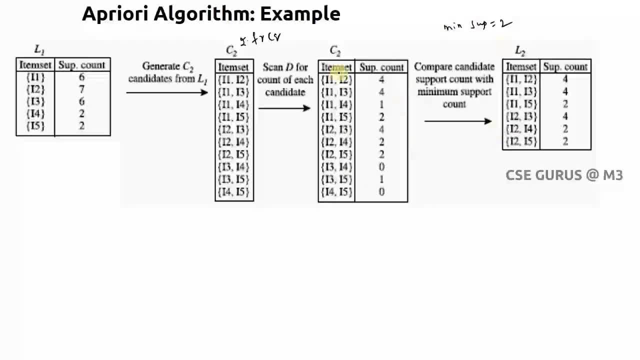 So minimum support count. I need to check How many item sets are satisfying. You can see here 1, 2.. This is not satisfying and this is not satisfying. This is not satisfying. This is also So I have to remove and I have to write the remaining, That is, we call it as L2.. After finding L2, you need to find what next, C3. So what is C3?? C3 means which is three frequent item set. So three frequent. 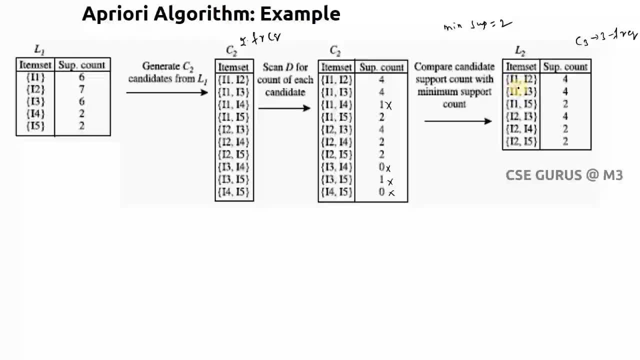 Means from this one. I need to find three frequent, three joints, Like in each line. I need to get only three items, Not four, not two. Okay, So if I make joints of these two, I1, I2, I1, I3. Can I combinedly say I1, I2, I3 if I join these two first two part, So this is a one joint: I1, I2, I1, I5.. Can I write it as I1, I2, I5?? 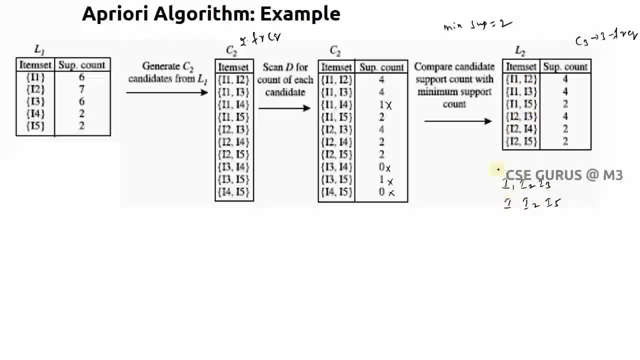 I1, I2, I2, I3.. So can I write it as I1, I2, I3?? Already written: I1, I2, I2, I4.. Can I write it as I1, I2, I4?? So, like this, we need to write I1, I2, I2, I5. If I consider So: I1, I2, I5.. Already I have written this. So, coming to this, I1, I3, I1, I5.. I1, I3, I5.. So I1, I3, I5.. Next, 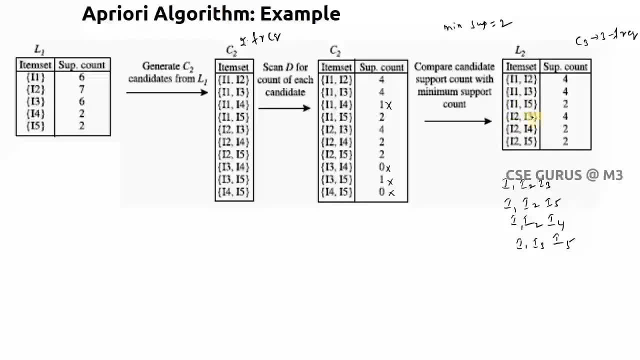 Next I2, I3. So can I write it as I1, I3, I2, I3? Means I1, I2, I3.. No See, every time if I take four, No One should be common. Then only I will get three joints. So next: I1, I3, I2, I4.. Now there is no common item. That's why I am getting I1, I3, I2, I4.. Four frequent items: We are not finding here four frequent. We require only three frequent. That's why we will ignore that part. So next: I1, I3, I2, I5.. That is I1, I2, I5. 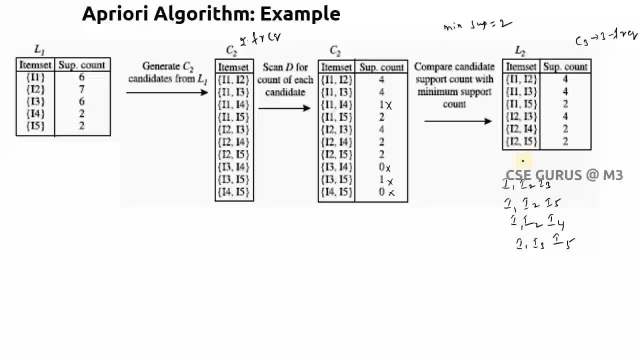 I3, I5. Again, four frequent, So we will not consider that one also. So I1, I5, I2, I3. Like this: if I consider What happens: I1, I2, I3, I5. I cannot consider I1, I5, I2, I4. So I1, I2, I4, I5. So I cannot consider I1, I5, I2, I5. So I1, I2, I5. I have to consider I2, I3, I2, I4.. I2, I3, I4. So that is a new one. 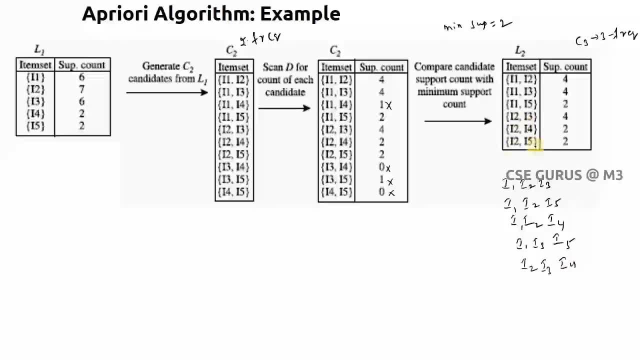 I am getting here Next I2, I3, I2, I5.. I2, I3, I5.. I will get I2, I3, I5. So like this, we need to consider I2, I4, I2, I5. So I2, I4, I5. So like this, all three frequent set, I need to get This. we call it as C3. Now what is the next step? Again for C2, we are getting scanning the database for support count. Again, find for support count of each one. That means the transactions: How many? 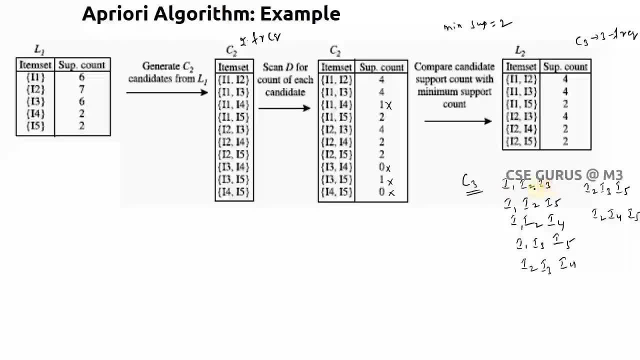 transactions. we are getting I2 and I1 and I3. All these three we need to get. So what is that support count? And for I1, I2, I5. Like this we need to find for all those things. If I find, I will. 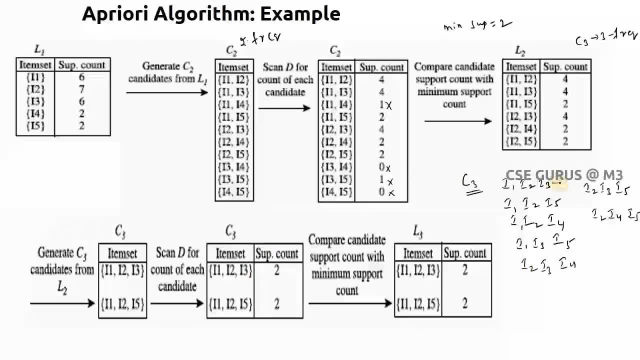 get all those things, but I1, I2, I3, I will get only two: I1, I2, I5. I will get two For the remaining, if you find you can find, you will get here the things which are less than two, So that 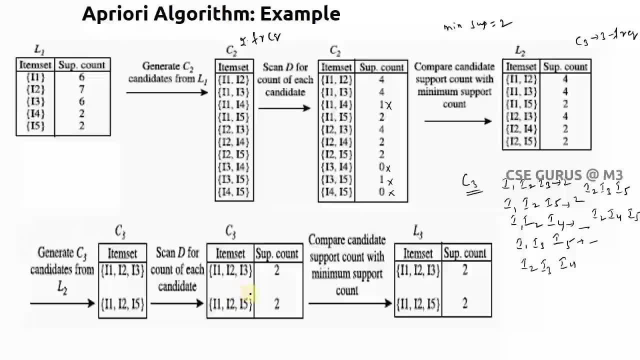 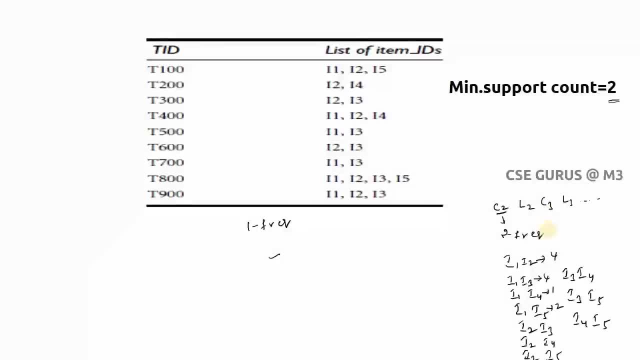 is why here directly those things are removed. Those are not frequent Item sets. So that is why, finally, I am writing, only two You can find for I1, I2, I4.. Let us suppose, if I check for I1, I2, I4, combination I1, I2, I4. One, Only one So, which is less than. 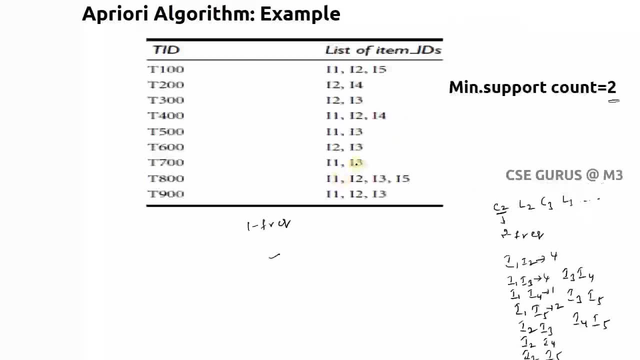 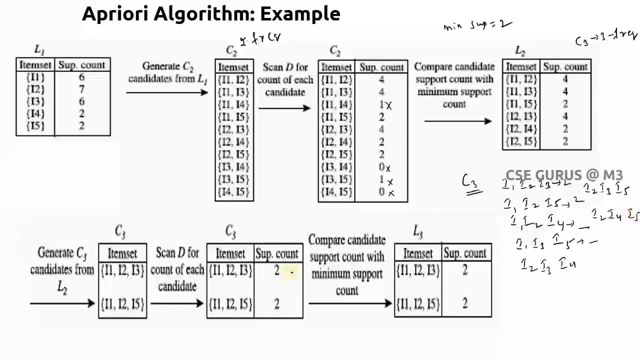 two. You can consider I1, I3, I5.. I1, I3, I5.. I1, I3, I1, I3, I5. Only one transaction, So like this we will get for the remaining item sets, which are less than two. That is why we are not taking 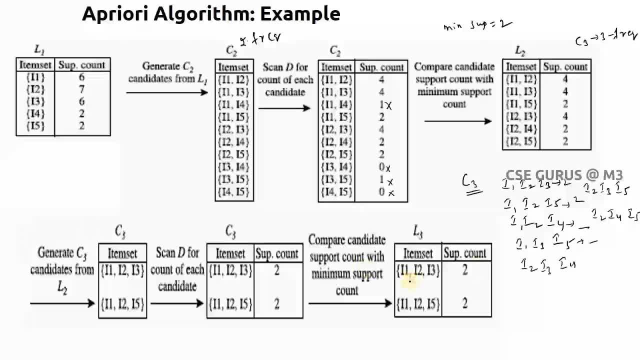 Because for L3, those things will be compared with support count which are not satisfying with the minimum support count. That is why we are neglecting those things. So, like this, we need to find L3. Now, after L3, you need to get C4. So what is this C4?? If I want to get, C4 means. 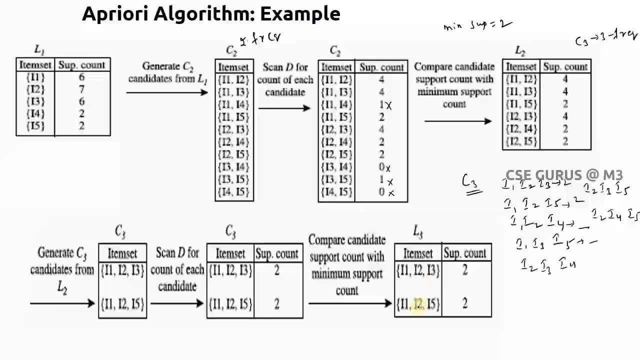 four frequent items. What are those four frequent item sets from L3?? So if only I have two sets. So if I combine these two I will get I1, I2, I3, I1, I2, I5.. So if I combine I will get only one thing, that is, I1, I2, I3, I5.. So only one thing I will get. 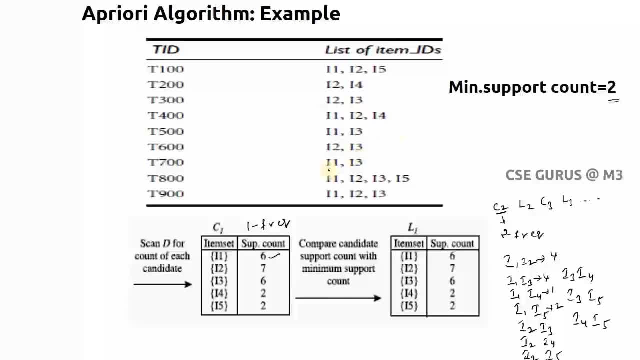 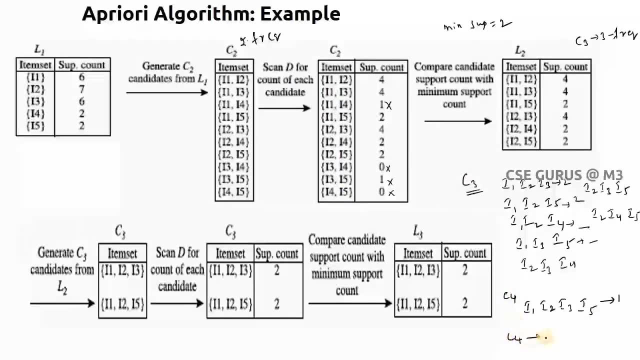 So if I go for the, what is that support count? What is the support count of I1, I2, I3, I5? Four you need to get, So if I consider I1, I2, I3, I5. So only one is there, So support count is one. 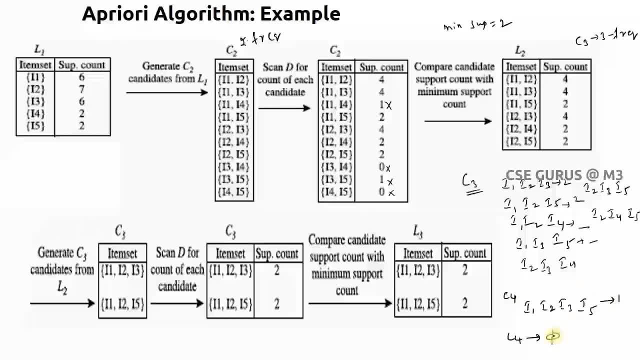 So this is C4. Now L4 will be empty. Why? Because it is only one transaction that is not satisfying. you will get empty set. you need to find all those things. if you don't get empty here, you need to find c5, next l5, like that you need to get now, after getting empty set. what is our solution? 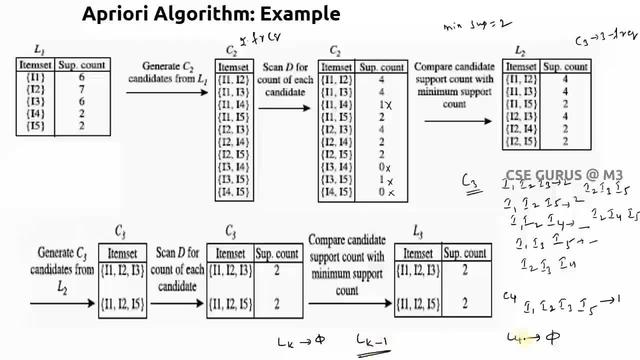 if you get l suffix k as empty set, now your solution will be l suffix k minus 1, so l4 is empty. that's why l3 is our solution. so what is that solution? two item sets are frequent. we are saying so. why we are doing all those things means finding frequent item sets. so what are our? 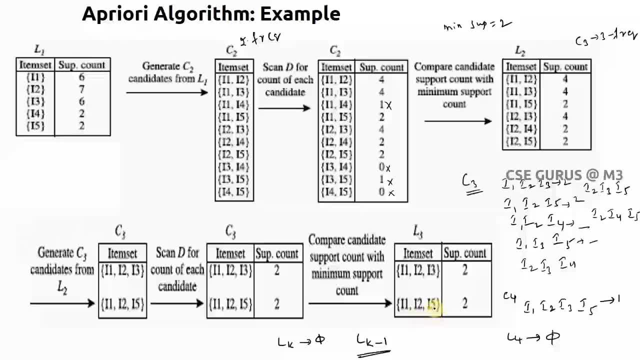 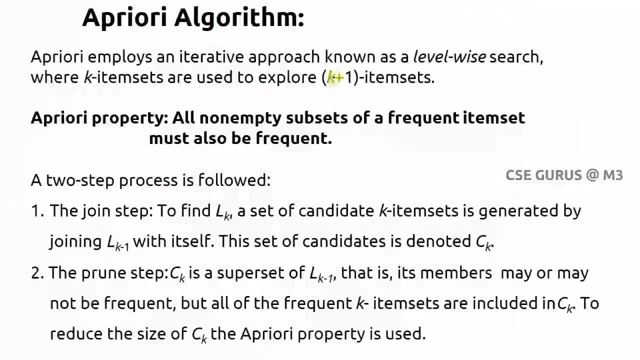 frequent item sets. one is i1, i2, i3 is one frequent item set. i1, i2, i5 is another frequent item set. that means those customers who are purchasing items i1, i2, i3 combinedly are more frequent. i1, i2, i5 is also one more frequent item set. like this we need to find now, if you go to the theory, 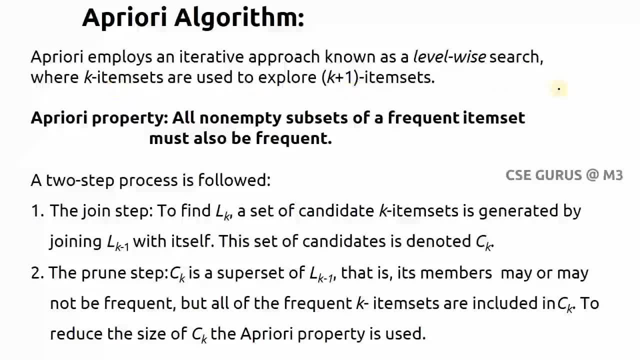 part apriori employs an iterative approach known as level wise set. so why we are saying it? as level wise set means where k item sets are used to explore k plus 1, that's what. so, in order to get l2, i am going for l1, i am checking for l1 in order to get l3. 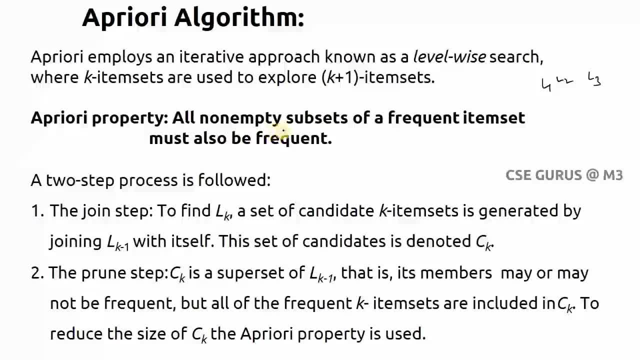 i am checking for l2 like this you are getting. so that's why you know where k item sets are used to explore k plus 1. so apriori property: all non-empty subsets of a frequent item sets must also be frequent. so what is the meaning of this one? all non-empty subsets of a frequent. what is? 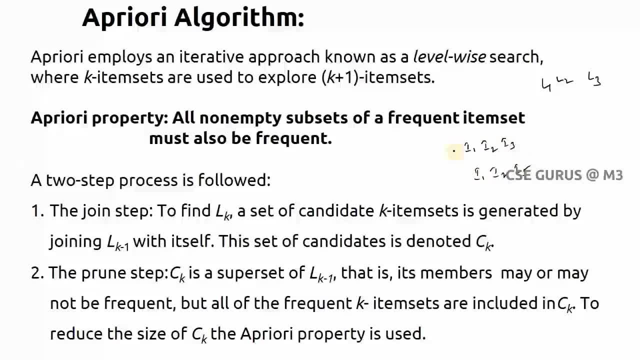 the frequent item set we are getting here: i1, i2, i3 is the one frequent item set. one more is i1, i2, i5. so if i say i1, i2, i3 is a frequent item set, there must be all non-empty subsets. what are the non-empty? 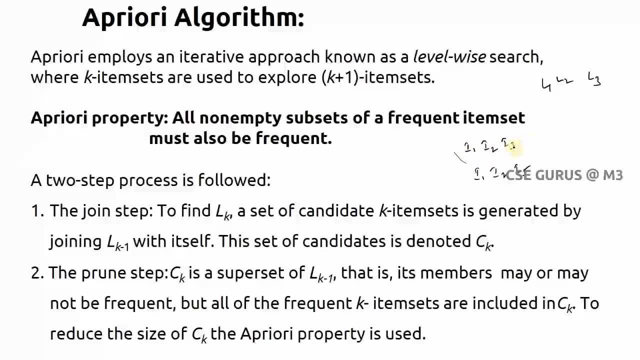 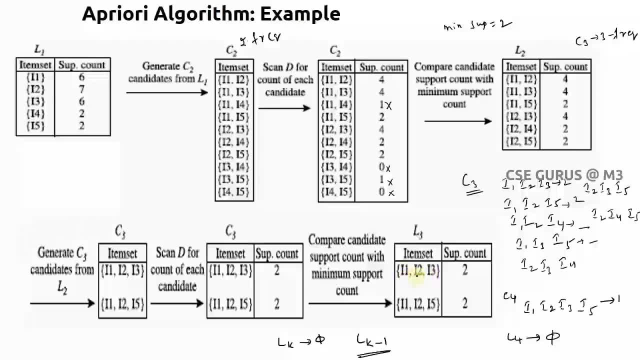 subsets: i1, i2, i1, i3, i2, i3 and also i1 separately, i2 separately, i3. so all these must be frequent. if you see this constraint. if i say i1, i2, i3 is a frequent item set. i1, i2, i3 is a frequent item set. 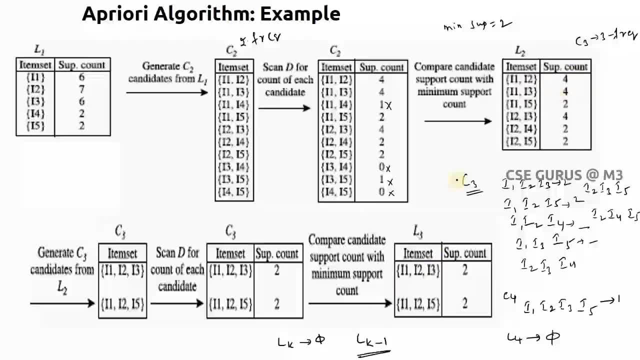 so all subsequent one is i1- i2. is it frequent? yes, if you can see here i1- i2 support count satisfying i1- i3. what is the support count for satisfying i2- i3? what is the support count for satisfying i1 separately? what is the support count 6 satisfying i2 separately. 7 satisfying. 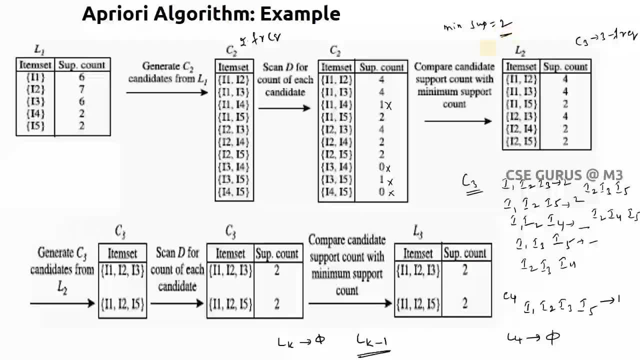 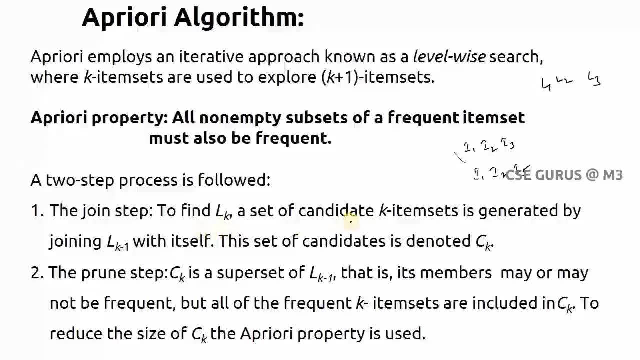 i3 separately satisfying, i1, i2, i3 combinedly satisfying. so all non-empty subsets must satisfy the minimum support constraint. that is why this property is called as a prairie property and that we are following and we are getting the answer. so join step and prune step. join, step means l suffix. 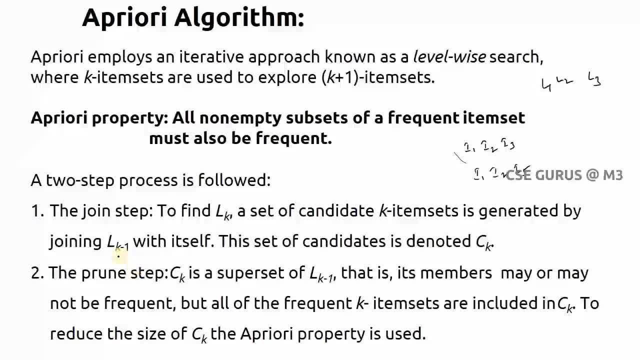 whatever we have taken, that is a join step. that means to find l suffix k- set of candidates, k item set generated by l suffix k minus 1, to get l3- l1 joined. l1 sets are joined to get l4- l3 sets are joined like that the sets of candidate is denoted by. whatever the result we are getting.